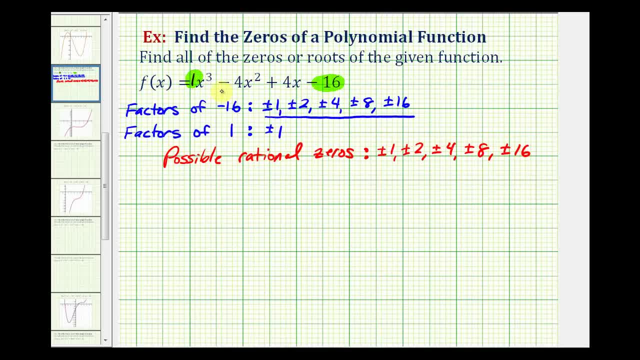 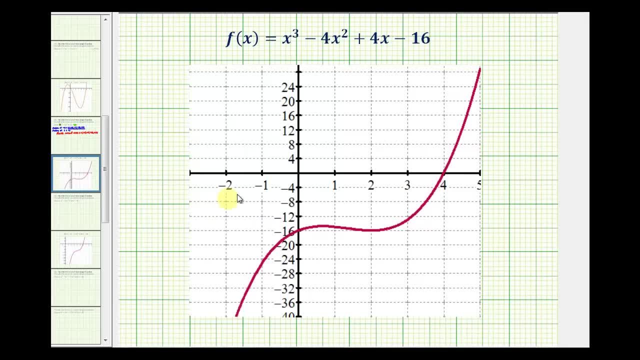 That means that the x intercepts of this function would be the real zeros of the function. So let's look at the graph of this function. We can see right away: this function only has one x intercept right here at positive four, which means the function would only have one real rational zero here at positive four. 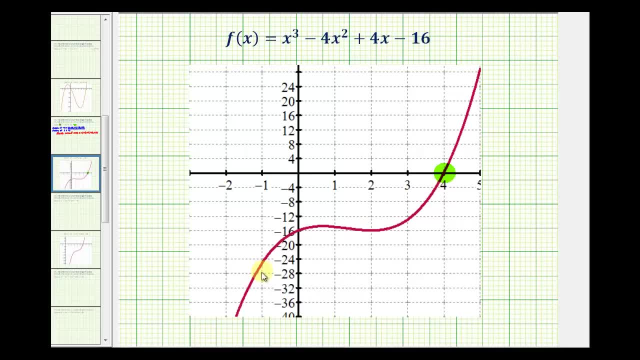 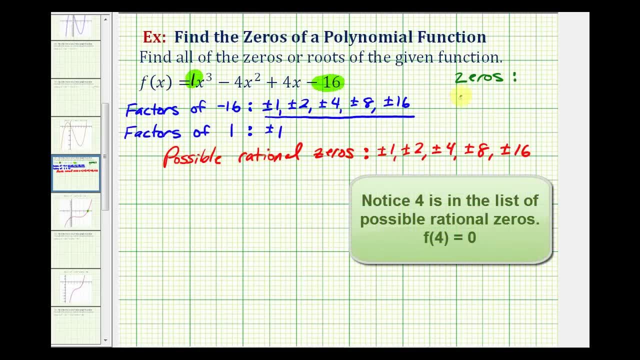 the other two zeros would be complex or imaginary zeros. So right now we know one of our zeros is x equals positive four. The next thing to remember is if x equals four is a zero, then x minus four would have to be a factor of this degree three polynomial, which means you can rewrite the function as f. 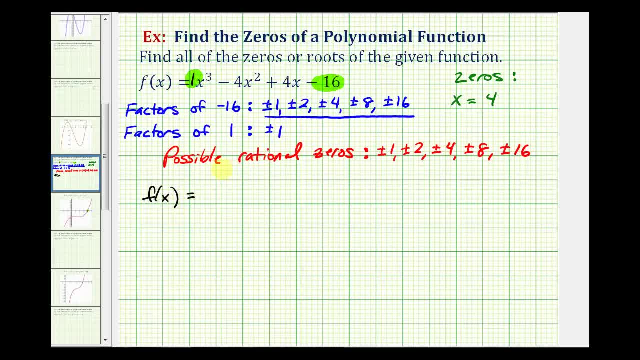 of x equals a factor of x, So x minus four. notice how this is a degree one, so the remaining factor would have to be a degree two factor, and to find this factor we can divide the original polynomial by x minus four or perform synthetic division using: x equals four. 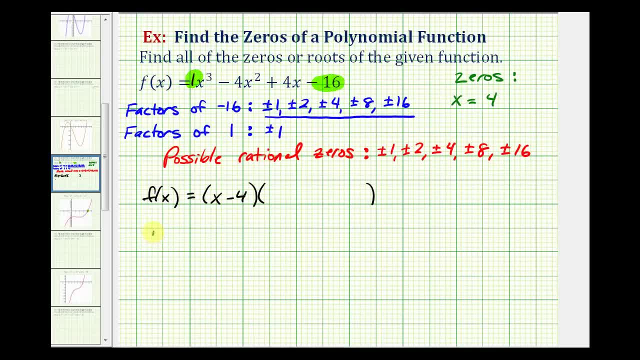 Let's go ahead and perform synthetic division. So we're going to use a four here. then we're going to list the coefficients of our polynomial, which are one negative four, four and negative 16.. Remember, because we're saying x minus four is a factor. 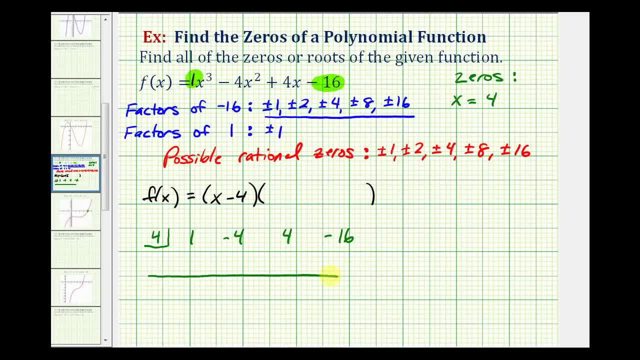 when we perform the synthetic division, the remainder must be zero. If it's not, we've made a mistake. So to perform synthetic division now, we bring the one down, multiply by four. four times one is four. we add this is zero. multiply by four. well, zero times four is zero. we add multiply by four. 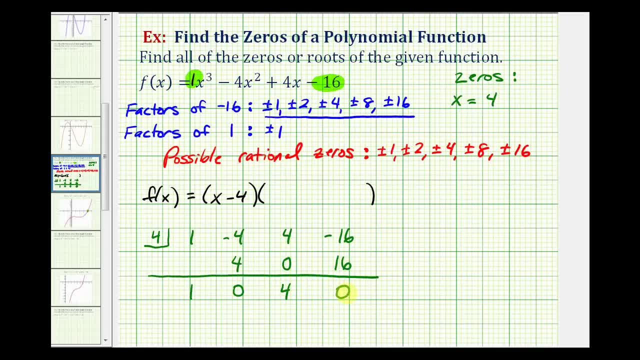 four times four is 16, and our remainder is zero, Which is good. So now we've confirmed that four is a zero of the function algebraically as well as graphically, but the results of this also gives us the remaining factor of our polynomial function. 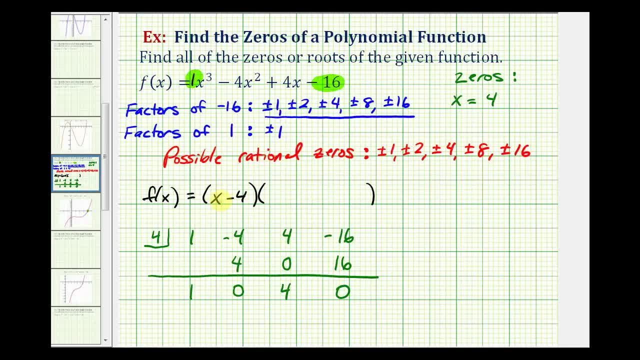 We started with a degree three polynomial. we divided by a degree one polynomial. therefore, our quotient would be a degree two polynomial. so this is the coefficient of the x squared term. So our factor is one x squared, or x squared plus zero x, which we can leave out. 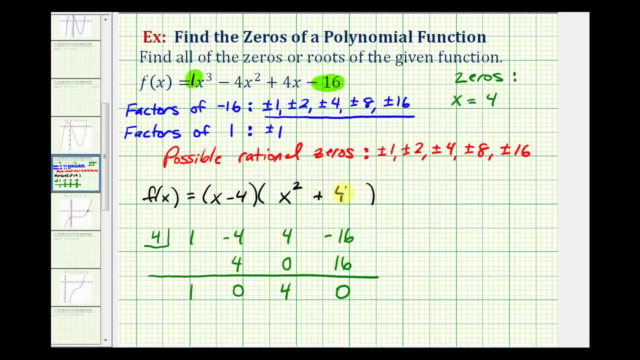 plus four, and again the remainder is zero. So these are the two factors of the original polynomial. Now we can find the remaining two complex zeros by finding the zeros of this factor here, since we already found the zero of this factor. So now we're going to set x squared plus four, equal to zero, and solve: 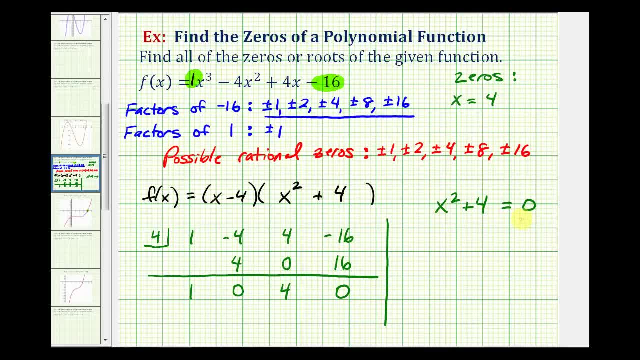 This is not factorable, so we could use the quadratic formula. but because we only have an x squared, we're going to use the quadratic formula and then we can isolate the x squared and then square root both sides of the equation. 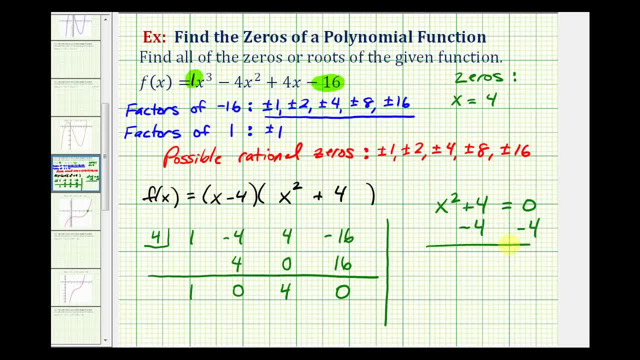 So let's go ahead and subtract four on both sides, So we have x squared equals negative four. so now we square root both sides of the equation so we'll have x equals. remember we'll have two solutions here. so we have plus or minus the square root of. to show this, I can write negative four. 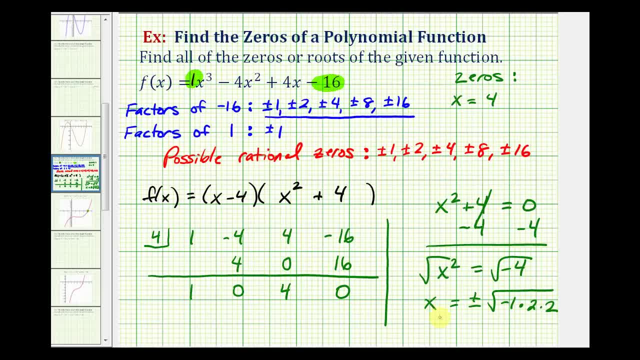 as negative one times two times two. So x is equal to plus or minus. well, the square root of negative one is i. the square root of two times two is. the square root of four is two. so we have: x equals plus or minus two i. so our remaining two zeros are imaginary. 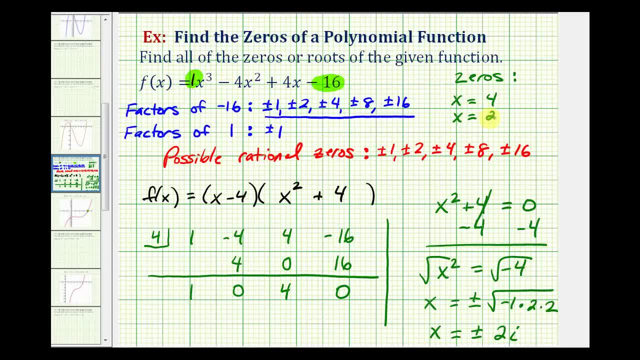 So our zeros are: x equals four, x equals two i and x equals negative two i, Which often we just write as plus or minus two i. So these are the zeros of the given value, given degree. three, polynomial function. Okay, I hope you found this helpful. 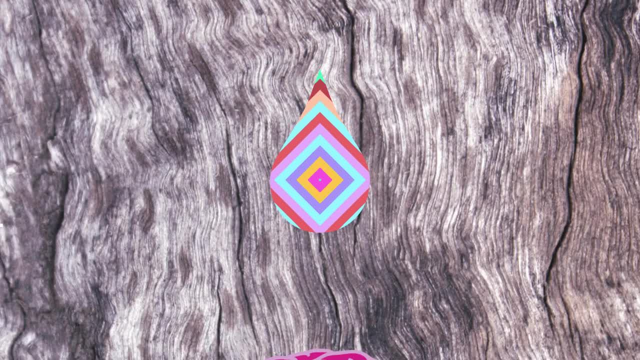 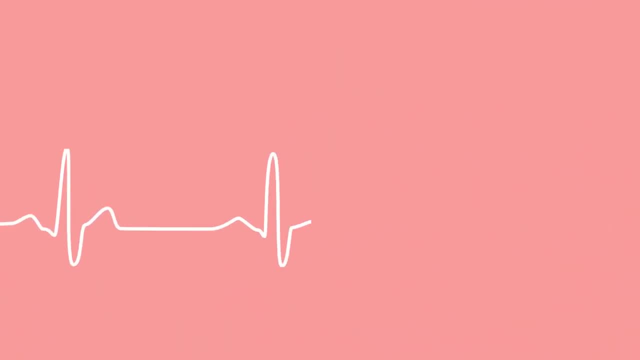 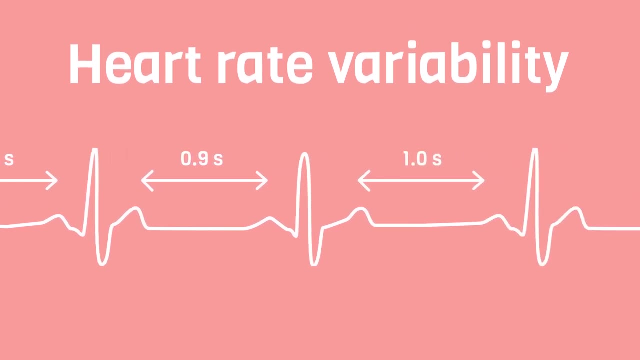 If you think your heart beats at a regular interval like a metronome, think again. We have a natural variability in the spacing between our heart beats. This phenomenon is called heart rate variability, and HRV for short. It says a lot about our bodily systems.